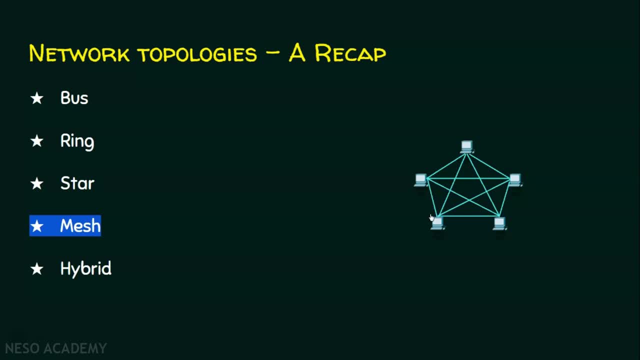 Coming to the mesh topology, every pair of nodes will have a dedicated line. If there is a node, every node will be connected with its other nodes through a dedicated link. And coming to the hybrid, a hybrid topology is a combination of one or more topologies. 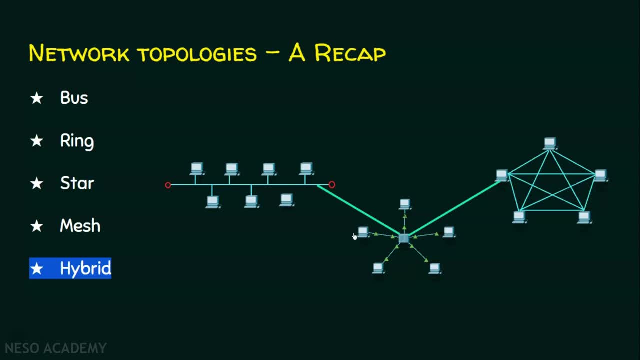 In this case, here is a bus topology which is connected to a star topology and in turn, this is connected to a mesh topology, and that is why we call this as a hybrid topology. Now we will move on to the questions. Question number one: 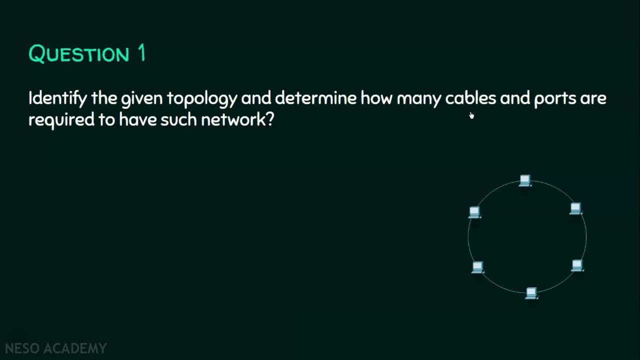 Identify the given topology and determine how many cables and ports are required to have such network. We are given with a topology and we have to identify what is this topology? And the answer is very simple: This is a ring topology. How many cables and ports are required to have such network? 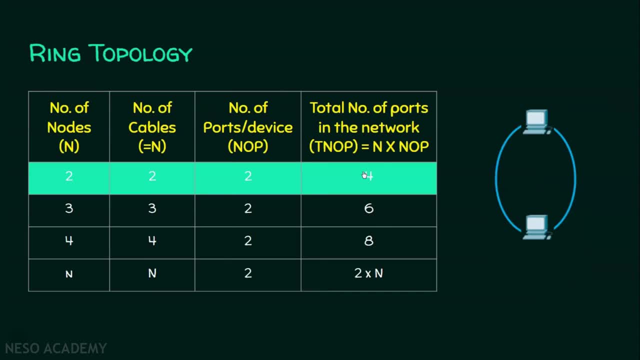 Let us formally solve this question In a ring topology. if there are two nodes, then we need two cables- This is cable one and this is cable two- And each node needs two ports. This is one port and this is port number two. 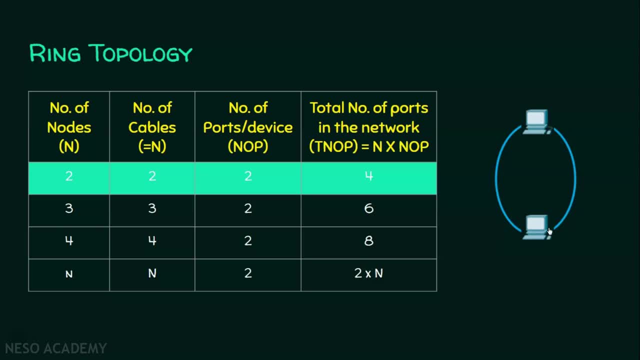 Similarly, this node also should have two ports: Port one and port two. So total of four ports are required. Each node must have two ports. So that is what is given here. So I have created a table like this where the number of nodes are listed. 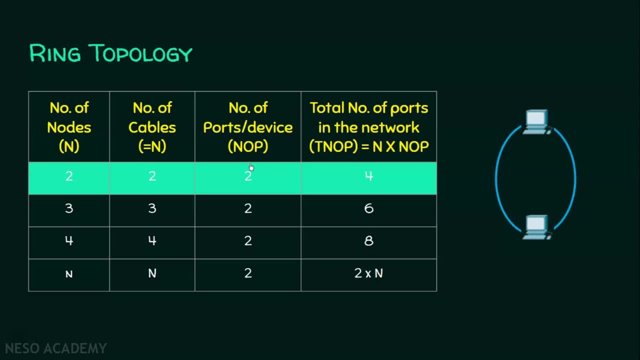 how many cables are required, the number of ports per device and the number of ports in the network. This is my own way of representation and if you want, you can use a different notation. If n is the number of node, if there are two nodes, 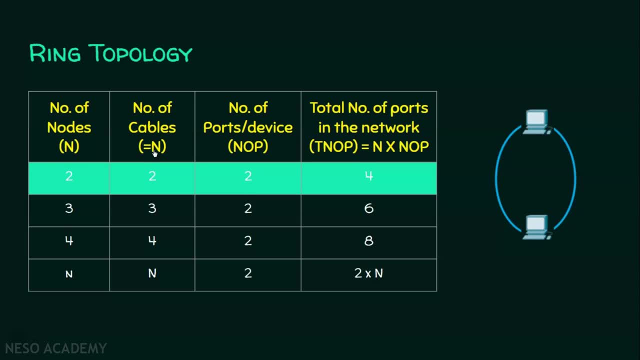 and we need two cables. So that is why we need two cables. So that is why I have used n. in both the cases, The number of nodes is equal to the number of cables in ring topology. This will not be the case for all topologies. 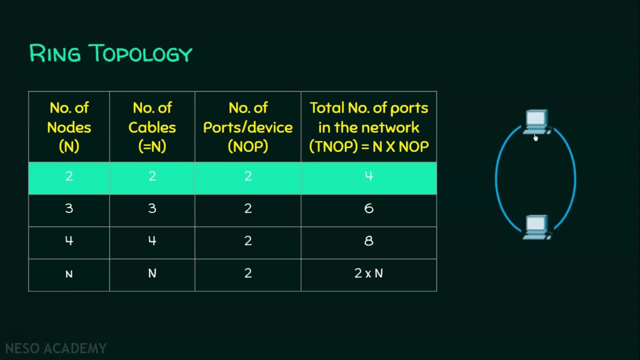 So if there are two nodes, we need two cables And each node must have two ports- and that is why I have mentioned two here- And a total there are four ports required. if the number of nodes are two, Some may have a question in their mind. 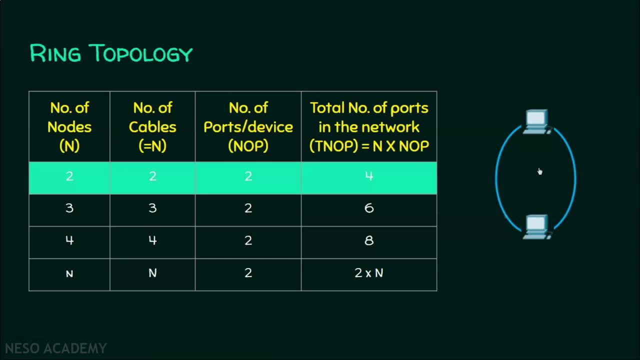 One cable is enough for this scenario. why do we need two cables? Actually, we aren't concerned about peer-to-peer networking, And this is a ring topology. A ring topology means that should be closed. It means there should be a cycle. 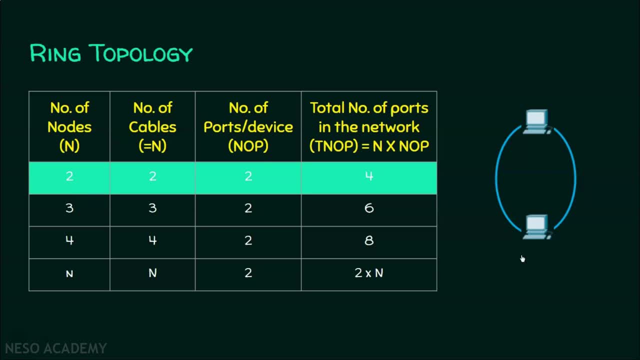 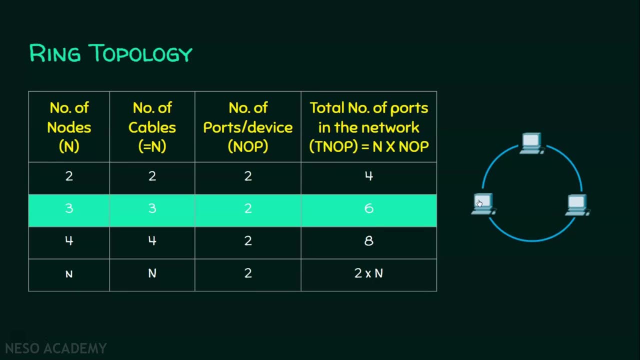 Now we will see a ring topology that involves three nodes. Now this is an example scenario that involves three nodes. If three nodes are involved, then obviously three cables are required. That is what I have mentioned here: Three nodes. it needs three cables. 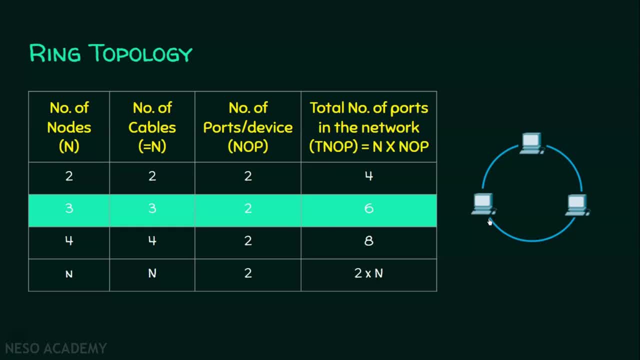 And each node must have two cables And each node must have two ports. Number of ports per device is equal to two, And therefore two into three, three nodes. Two into three is equal to six. A total of six ports are there in the network. 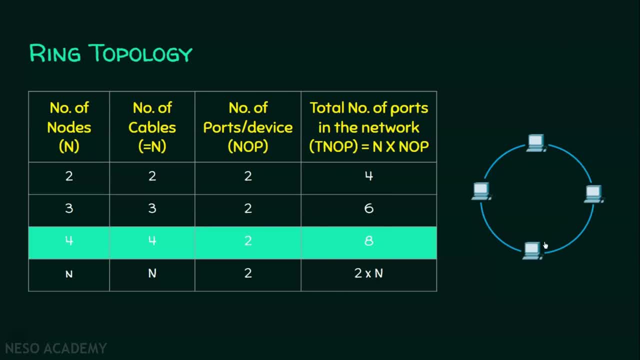 Now we will see if the number of nodes is four. If there are four nodes in a ring topology, then four cables are required, Cable one, two, three and four, And each node must have two ports And the total of two, two, two, two cables. 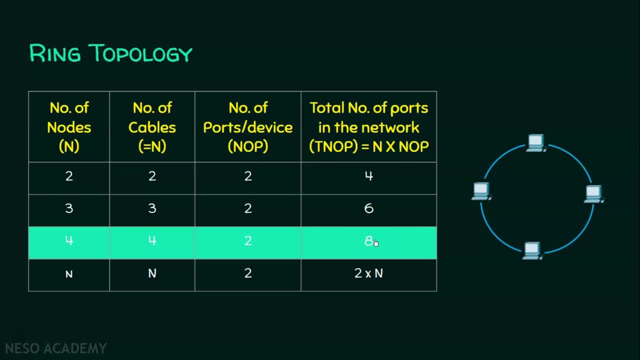 So two plus two plus two plus two, so a total of eight ports are required If there are hundred nodes in a ring topology. and it is very difficult to manually draw hundred nodes and solve it, So we need a formula to do this. 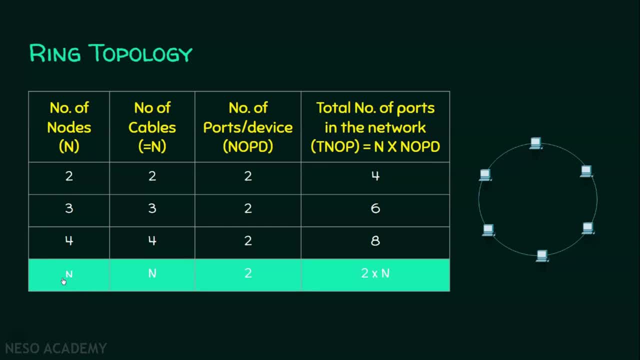 The generic formula is: if there are n nodes, then we need n cables. Each node must have two ports. therefore the number of ports, total number of ports in the network, is equal to two into n. So I have given a formula. 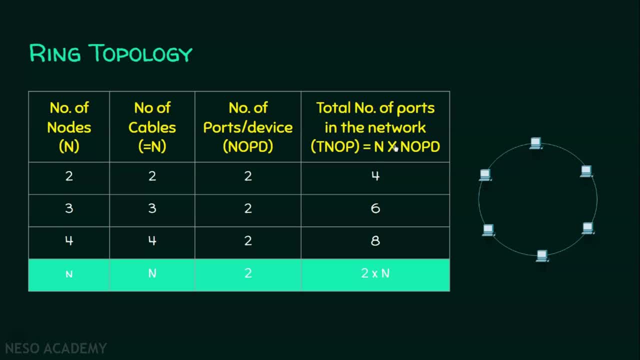 total number of ports is equal to number of nodes into number of ports per device. This is number of ports per device. As far as ring topology is concerned, number of ports per device will always be two only, So it is fixed as two. 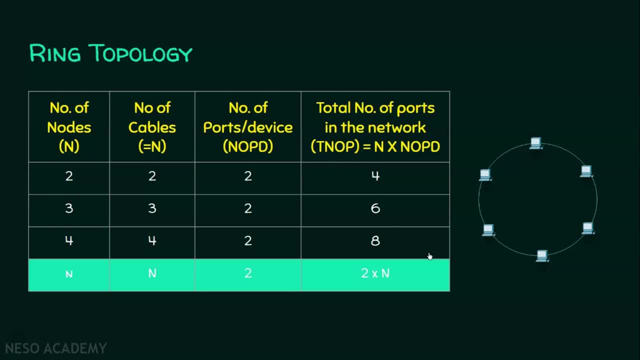 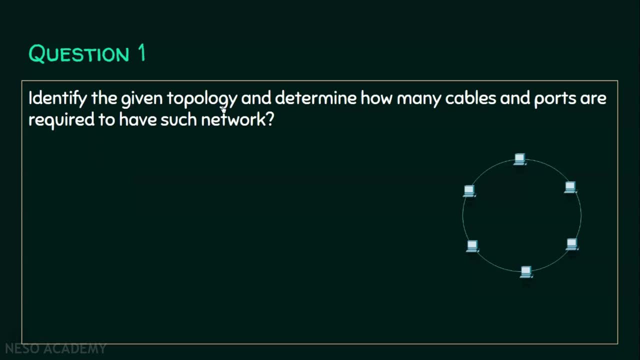 and two into number of ports will give you the total number of ports. We will revisit this question again. Identify the given topology. We have identified this. It is a ring topology And now we will determine how many cables and ports are required to have such network. 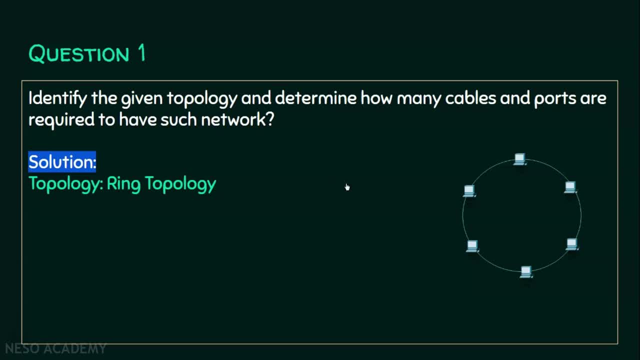 And the solution to this is: it is a ring topology and here the number of nodes are six. This is one, two, three, four, five, six. So there are six nodes, and that is why I have mentioned, as n is equal to six. 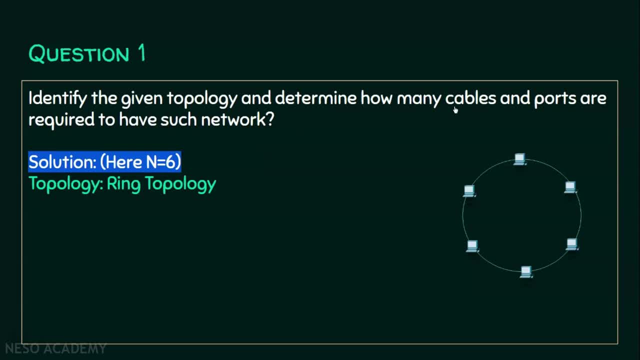 If n is equal to six, then the number of cables that are required is also six. We know that if n is the number of nodes, then the number of cables that are required is also six. Therefore, we need six cables in a ring topology. 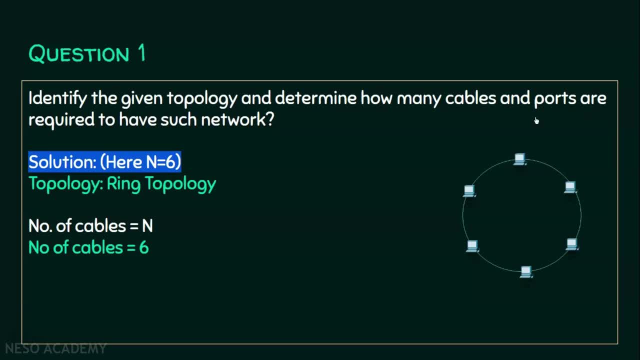 for this topology. Now we will see how many ports are required. We know very well the total number of ports is equal to the number of nodes into number of nodes per device. We know number of ports per device is equal to two. 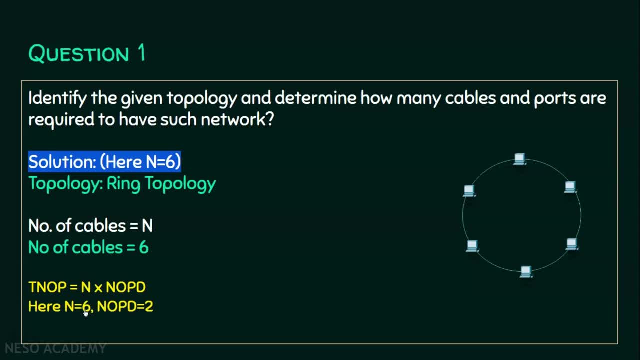 and the number of nodes is equal to six. So n is equal to six and number of ports per device is equal to two. So when we solve, the total number of ports is equal to two and the number of ports per device is equal to two. So when we solve, 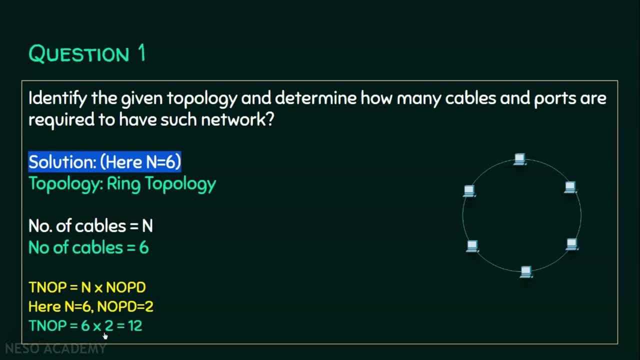 the total number of ports per device is equal to two and the number of ports per device is equal to two. So, when we solve, the total number of ports in the network is equal to six into two, which is equal to twelve. 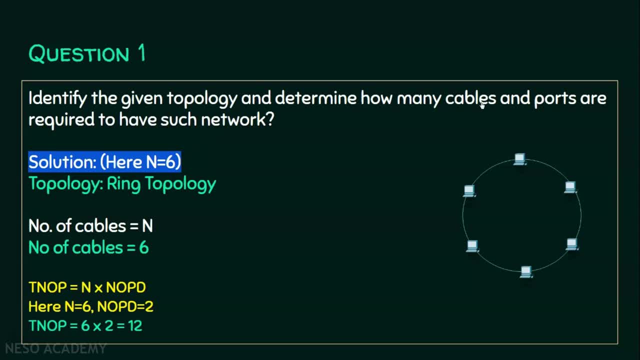 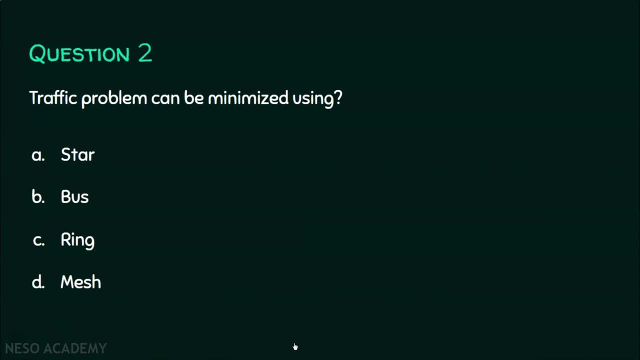 The answer for this question is: it is a ring topology and it needs six cables and total twelve ports are there in this network. Now we will move on to question number two. Traffic problem can be minimized using A star B bus. 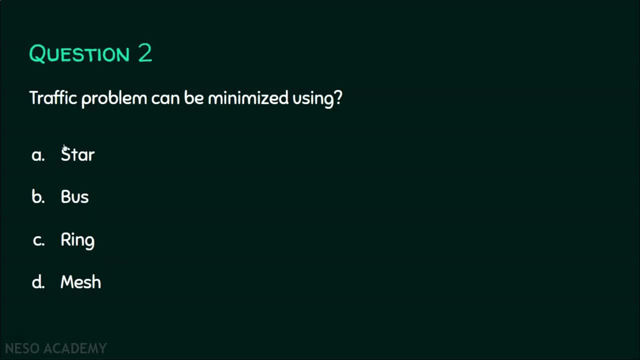 C ring and D mesh topology. We have to identify in which topology there is minimal traffic. This is a star topology, this is a bus topology, this is a ring topology and here is the mesh topology. First we will check whether there is a traffic problem in star topology. 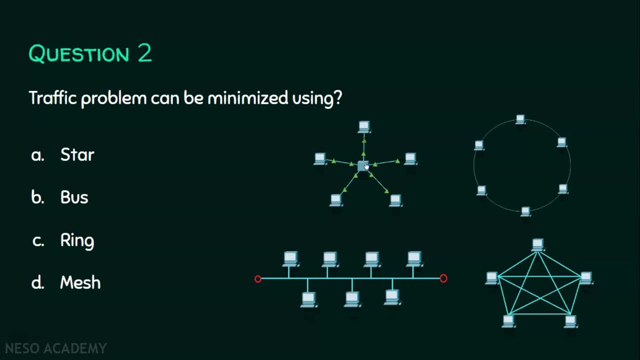 In star topology, all nodes are going to send traffic or data to the central hub. Obviously, traffic is high in the central node, So star topology is not the answer. And coming to the bus topology, we know very well that it is depending on the common transmission medium. 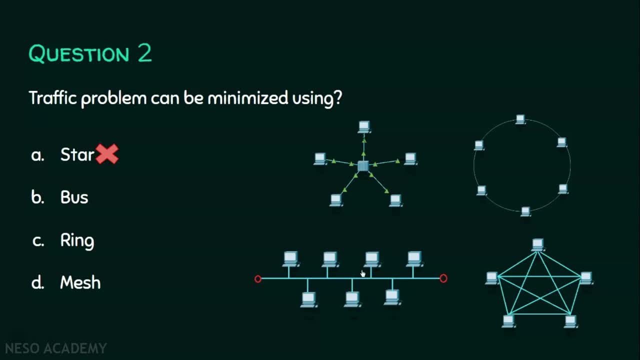 and all nodes are going to use this common transmission medium And it is a bidirectional communication too. So traffic problem is there in bus topology also. So this is also not the answer. And coming to the ring topology, we know very well that 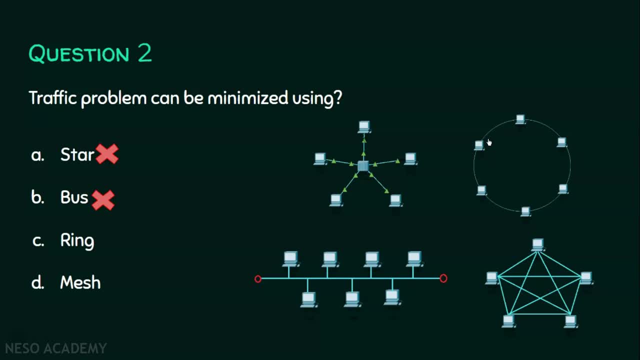 it is a unidirectional communication and all traffic will be in this direction. only Suppose if this is going to send some data to this device. it cannot send this way, because if the traffic pattern is like this, then it will not send this way. 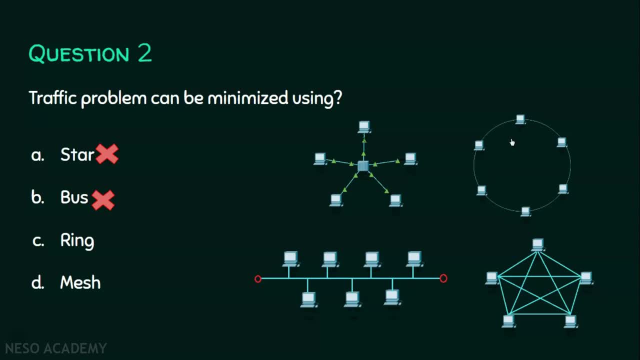 Because if the traffic pattern is like this, then it has to send in this way only. Similarly, all devices will be sending their data in this pattern only. So traffic problem cannot be minimized using ring topology And coming to the mesh topology. 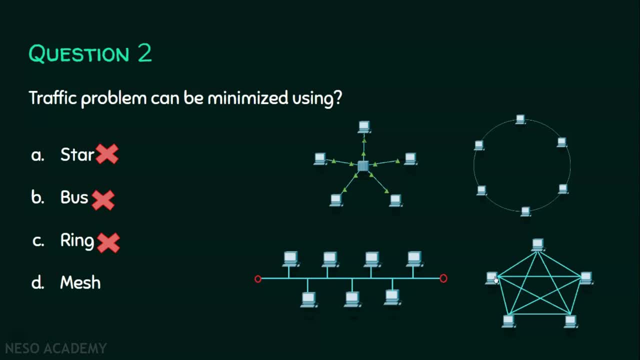 every pair of nodes have a separate line or a dedicated line or a dedicated channel. Since every pair of node has a dedicated link, so there is no traffic problem in this case, Suppose if this wants to send some data to this node. 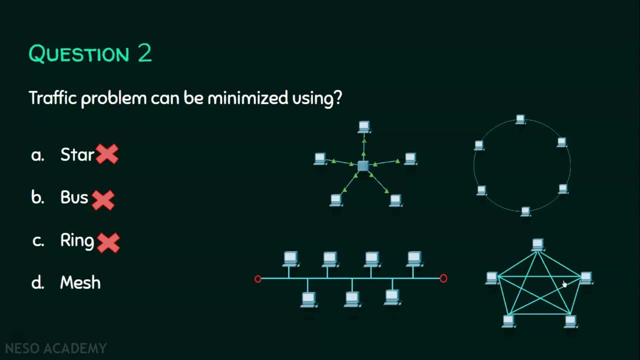 so it uses this line, and this is a dedicated line that is exclusively for these two nodes, And if this node wants to send some data to this node, it uses this dedicated line. So the answer for the question is: traffic problem can be minimized using mesh topology. 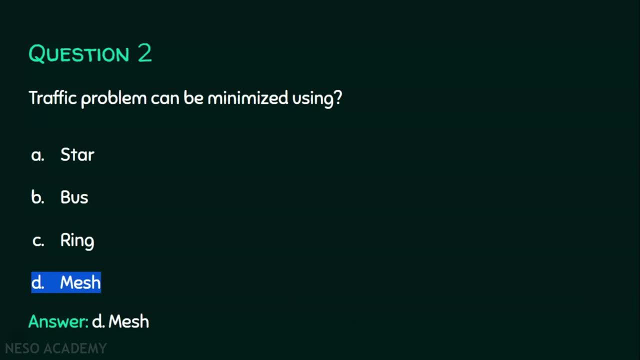 The answer is mesh topology. Now we will see question number three: How many ports and cables are required for a star topology? In a star topology there will be a central node connected to the central node. So if we observe, we will say there are one, two, three, four, five ports. 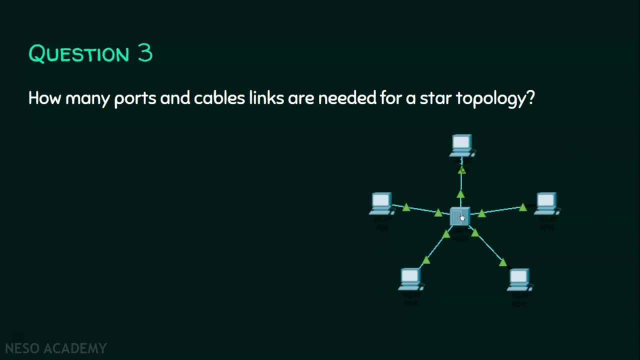 If there are five devices, we will say there are five ports. But that is wrong, because this central device also should have a port. If we are concerned about only particular node, then it needs only one port, But in the entire scenario there are ten ports. 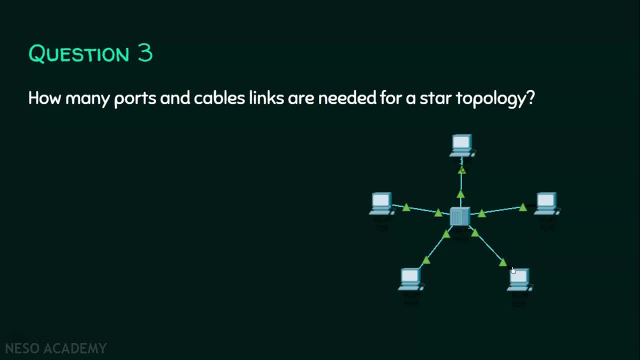 One, two, three, four, five, six, seven, eight nine ten. One two, three, four, five, six, seven, eight nine ten. One, two, three, four, five, six, seven nine ten. 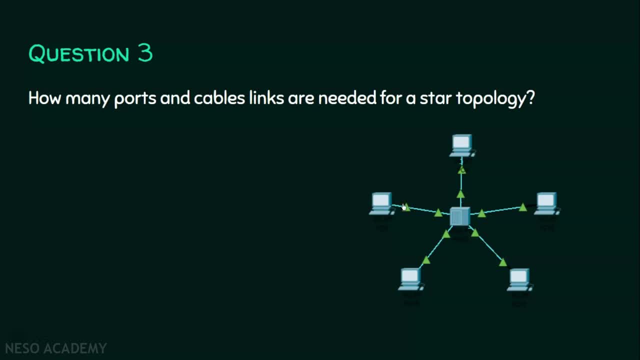 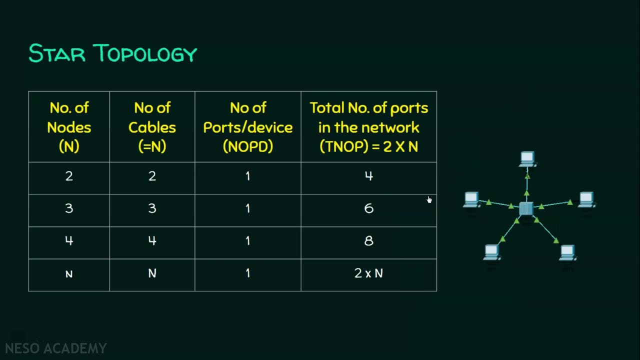 One, two, three, four, five, six, seven, eight, nine, ten. So there are ten ports and there are five cables. It is very easy to solve it if the scenario involves a very small number of nodes, But we have to formally solve it. 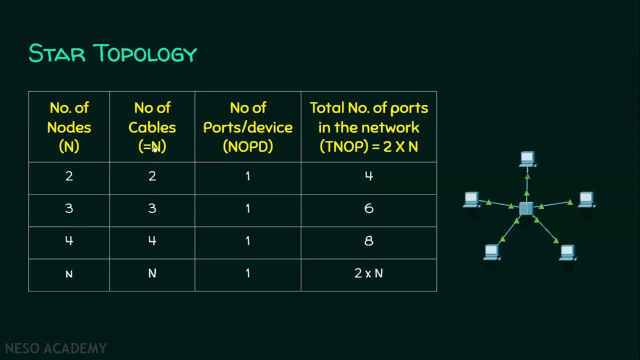 If n represents the number of nodes, then the same number of cables are required. We can evidence this example: One, two, three, four, five nodes and one, two, three, four and five cables. So if it uses only two nodes, it uses two cables. 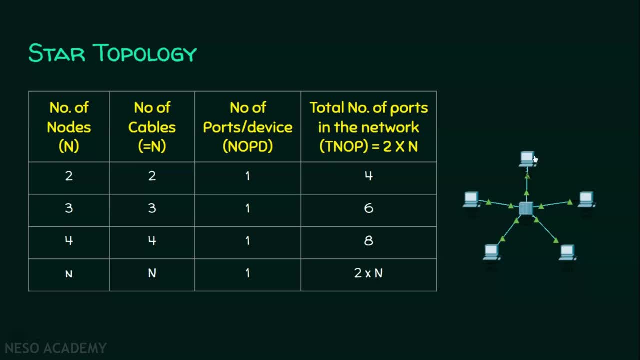 Similarly, three nodes means three cables, And each node will have one port. So the number of ports will be one. But do remember we have to focus on this part also. So I have given a generic formula. total number of ports is equal to two into n. 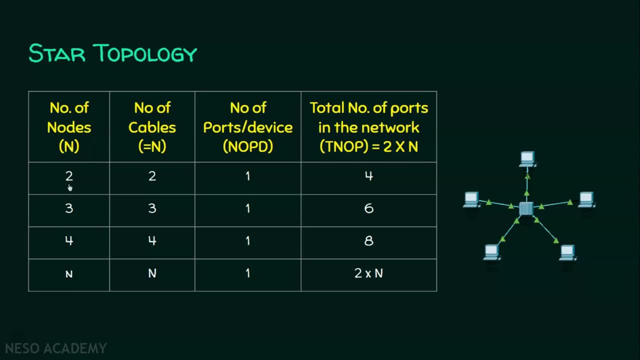 where n is the number of nodes. If our network involves only two nodes, we need two cables and we know very well that every device will have two cables. and we know very well that every device will have two cables. So if we have one port, 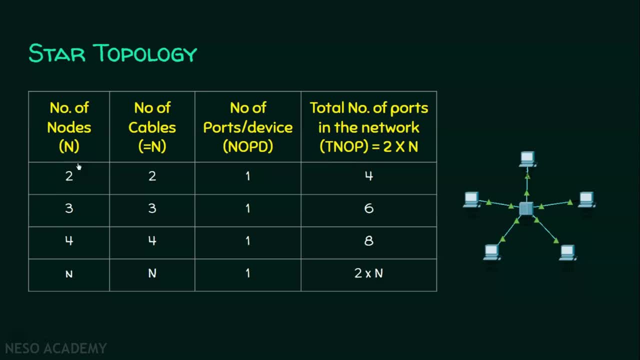 the total number of ports will be two into n. In this case, n is equal to two, So two into two is equal to four. If three nodes are involved, we need three cables and every device will have one port only, And total number of ports is equal to two into three. 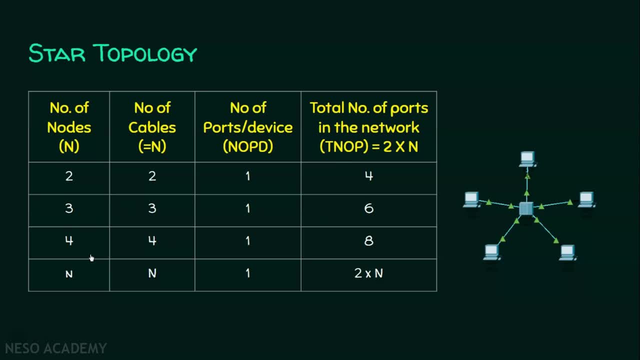 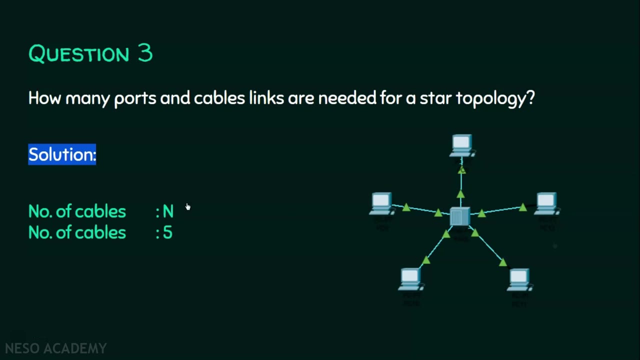 which is equal to six. If there are four nodes, then there will be eight ports. If n nodes are there, two into n is the total number of ports. The answer to question three is: if there are n nodes and we need n cables. 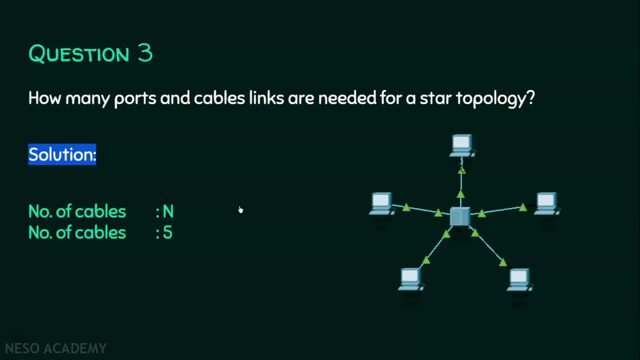 In this case, n is equal to five, so we need five cables And the number of ports is equal to two into n, where n is equal to five in this case. so two into five, which is equal to ten, The number of ports. ten means 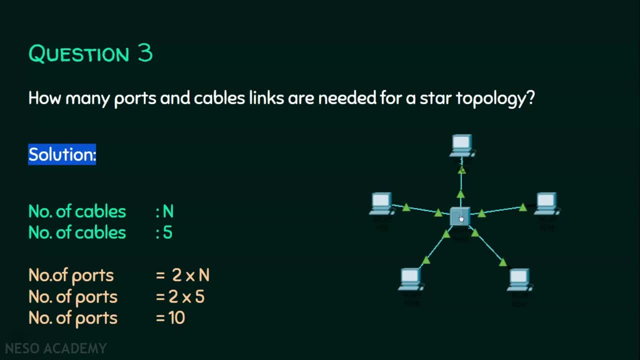 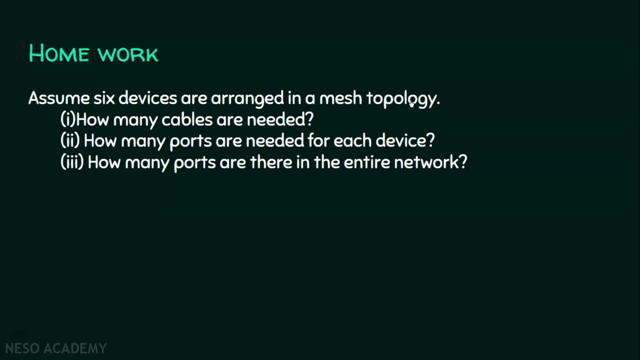 the ports involved in the n devices as well as the intermediary devices. There is a homework problem for you. Assume six devices are arranged in a mesh topology. We are required to find how many cables are needed, how many ports are needed for each device. 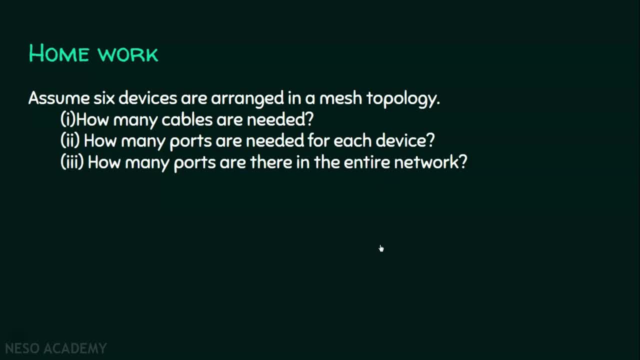 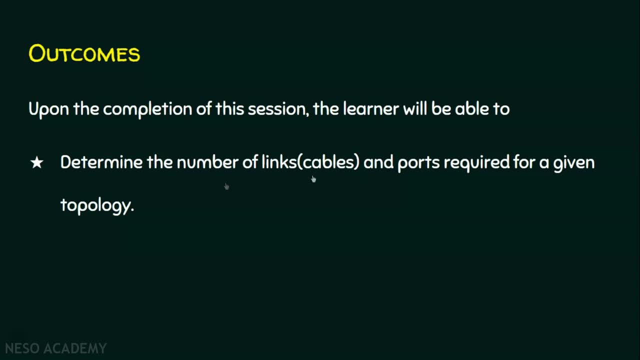 how many ports are there in the entire network? Derive a formula and post your answers in the comment section. I hope now we will be able to determine the number of cables or links and the number of ports required for a given topology. I hope the session is informative. 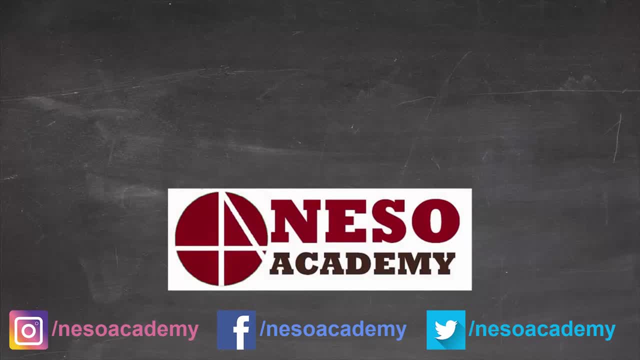 and thank you for watching. Thank you for watching.